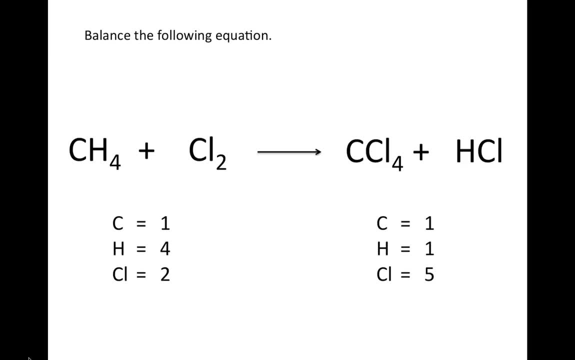 atom and five chlorine atoms. Now looking at this equation, because we have one carbon atom on the reactant side and one carbon atom on the product side, carbon is already balanced, So our next step would be to balance the number of hydrogen atoms, and I'm choosing to start. 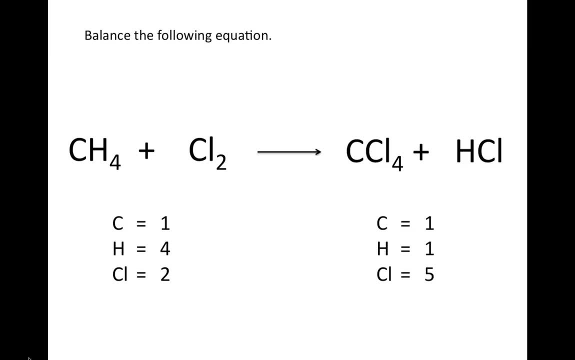 with hydrogen, because hydrogen occurs in one compound on the reactant side- CH4, and one compound on the product side, HCl. In order to balance the number of hydrogens on the product side, we're going to want to put a 4 coefficient in front of HCl. 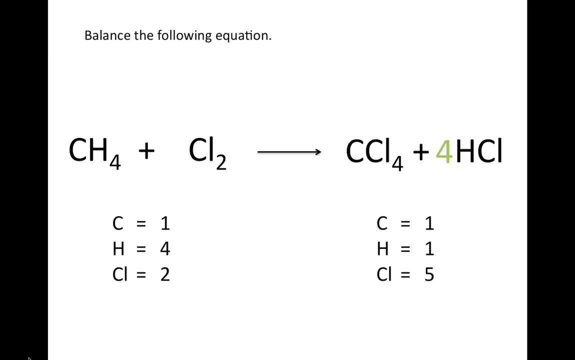 Remember, we can only add coefficients, we can never change subscripts. Now, if we count up the number of each type of atom we have on both sides, you'll see that we still have one carbon atom on both the reactant side and the product side. but 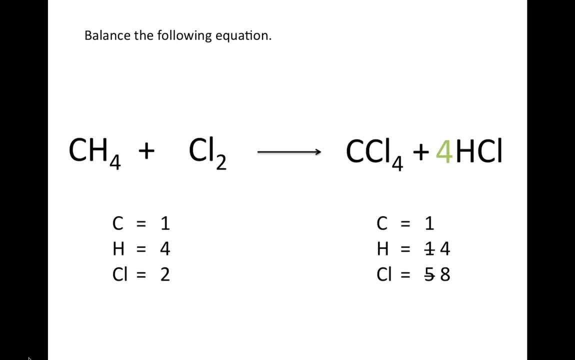 now we have four hydrogen atoms on the reactant side and four hydrogen atoms on the product side. But by putting a 4 coefficient in front of HCl on our product side, we not only have increased the number of hydrogen atoms on our product side, but we've increased the 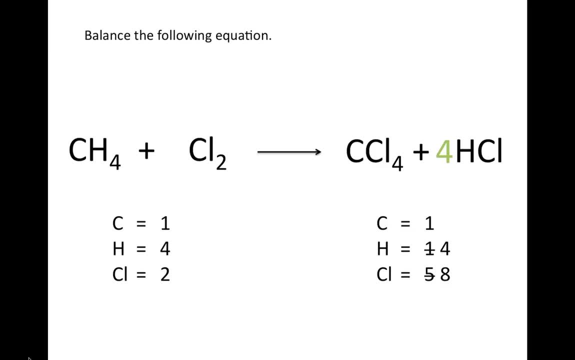 number of chlorine atoms on our product side as well. So if we look at our new total, We still have one carbon atom on our product side, but we now have four hydrogen atoms and we now have eight total chlorine atoms: Four from the CCl4 that we had to begin with and four from our four molecules of HCl. 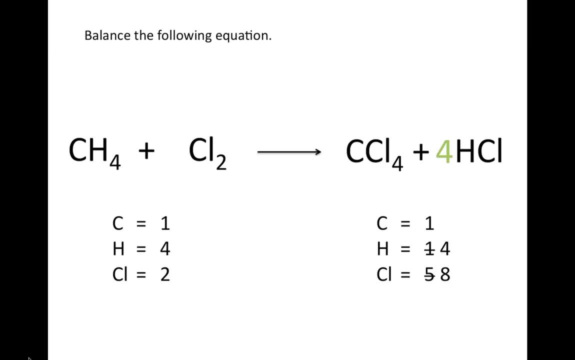 If we compare the types and numbers of atoms that we have on the reactant side and the product side now, we'll see that we still have one carbon atom on each side. We have four hydrogen atoms on each side, But on our product side we have eight chlorine atoms and on our reactant side we only have 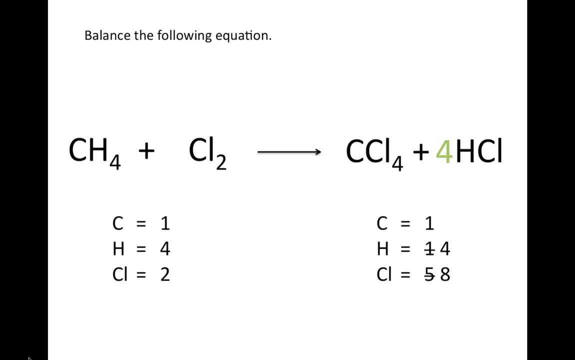 two chlorine atoms. So in order to balance our chlorine, we're going to add a four coefficient in front of our Cl2 molecule, And if we have four molecules of Cl2, that now means that we have eight chlorine atoms on our reactant side. 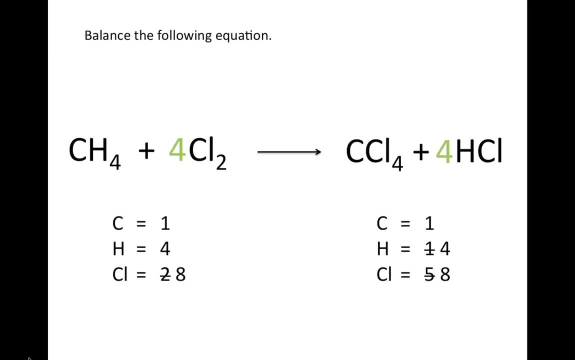 And remember, I chose to add four as the coefficient in front of Cl2, because each molecule of Cl2 has two chlorine atoms. So if I have four molecules of Cl2, that gives me a total of eight chlorine atoms, which I found just by multiplying four times two. 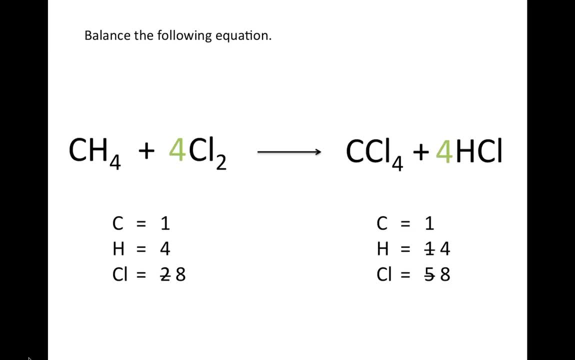 And now that we have the same number of each type of atom on the left side of our reaction arrow and the right side of our reaction arrow, we can consider this reaction correctly balanced. And after you feel that you've correctly balanced your chemical equation, the last thing to 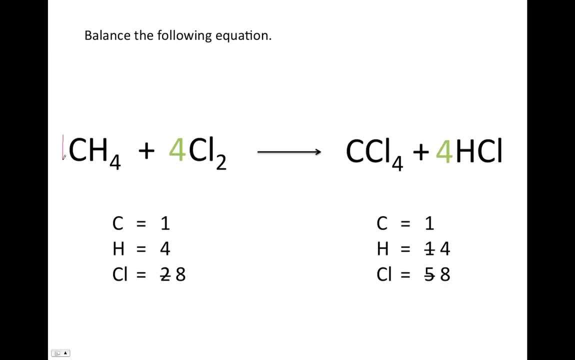 check is that your coefficients, which would be a one- here We don't typically write four, one and four are in their lowest ratio. Having coefficients that aren't in the lowest ratio does not make the chemical equation incorrect, but typically instructors and classes are looking for the lowest ratio when. 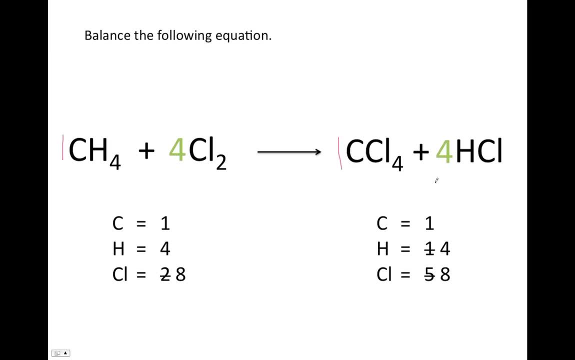 considering a balanced equation, And typically, when balancing your equation using this method, you will come up with the lowest ratio. But it's just one more thing to keep in mind. Let's take a look at another example. Again, I'm going to start by taking inventory of how many of each type of atom I have on. 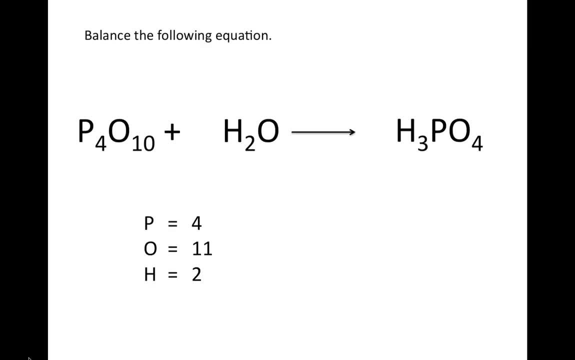 the reactant side and the product side. On the reactant side, I have four phosphorus atoms, 11 oxygen atoms, 10 from the molecule P4O10, and one from the molecule H2O, giving me a total of 11.. 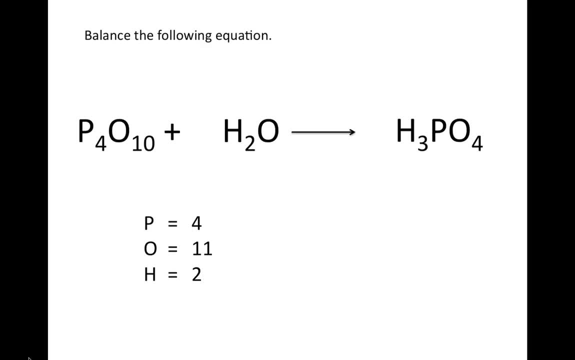 And two hydrogen atoms, And two hydrogen atoms And two hydrogen atoms. On the product side, I have one phosphorus atom, four oxygen atoms and three hydrogen atoms. Let's start by balancing the number of phosphorus atoms- And again I'm choosing phosphorus because it occurs in one compound- on the reactant. 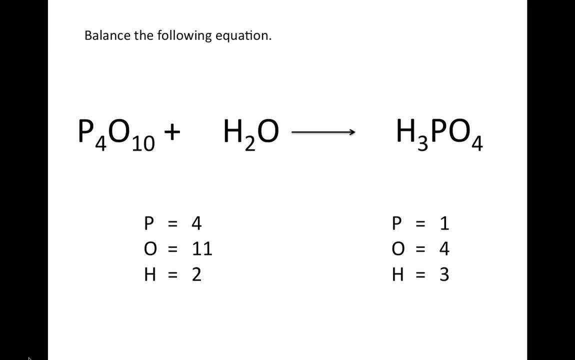 side and one compound on the product side, And it seems to be. if you follow this method, it'll make balancing the reaction a little bit easier. I'm going to really balance whichever type of atom you prefer first, Because I have four phosphorus atoms on my reactant side, I know that I need four phosphorus. 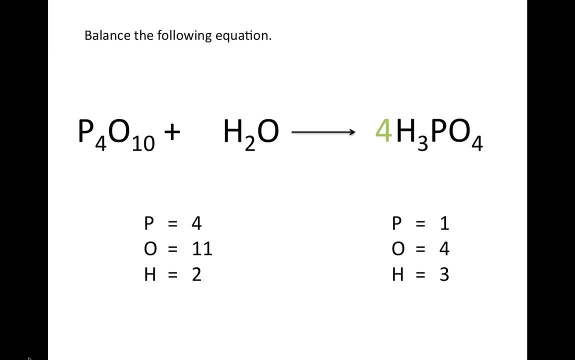 atoms on my product side, And because I can't change the subscripts of any atom, I have to add my four as a coefficient in front of the molecule H3PO4.. By adding four as my coefficient in front of H3PO4, I have now changed the number of 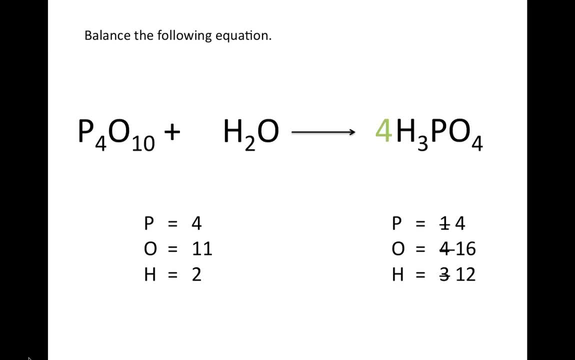 but I've also changed the number of oxygen atoms and hydrogen atoms. So to determine the number of oxygen atoms I now have on the product side, I multiply the coefficient by the subscript on the oxygen, which gives me 16.. And to determine the number of hydrogen atoms I have on the product side, 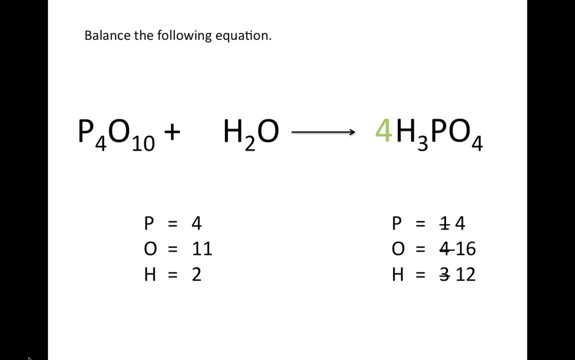 I multiply the coefficient by the subscript on the hydrogen, which gives me 12 hydrogen atoms. Now that I've balanced the number of phosphorus atoms on the reactants and product side, I'm going to balance the number of hydrogen atoms next. So, using the new number of atoms that I've calculated, I have 12 hydrogen atoms on my product side. 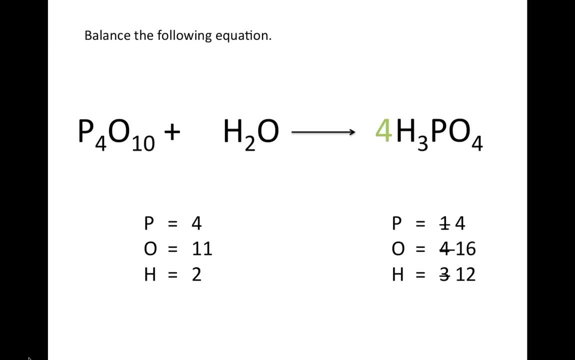 In order to give me 12 hydrogen atoms on my reactant side, I know that I'm going to need to add 6 as a coefficient in front of H2O, So 6 times the subscript on H, which is 2, now gives me 12 hydrogen atoms on my reactant side. 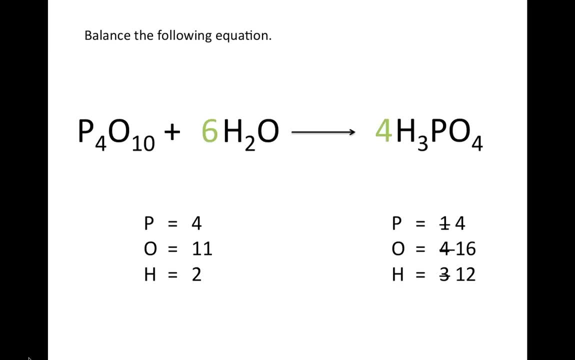 But again, because I've calculated the number of hydrogen atoms on the product side, I put a coefficient in front of the entire molecule. I've not only changed the number of hydrogens on the reactant side, but I've also changed the number of oxygens. 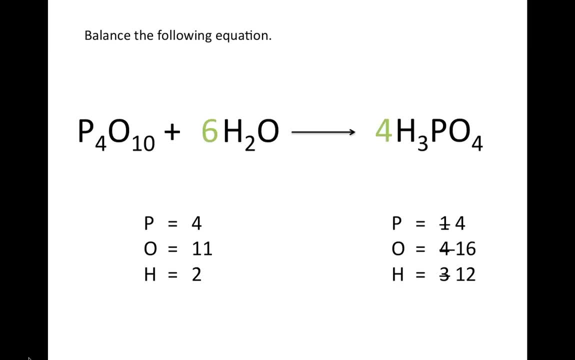 I now have my original 10 oxygens from the compound P4O10, but I have an additional 6 oxygens because I have 6 H2O molecules, which gives me a total of 16.. Now you can see, in this case, balancing our hydrogen automatically balanced the number of oxygen atoms. 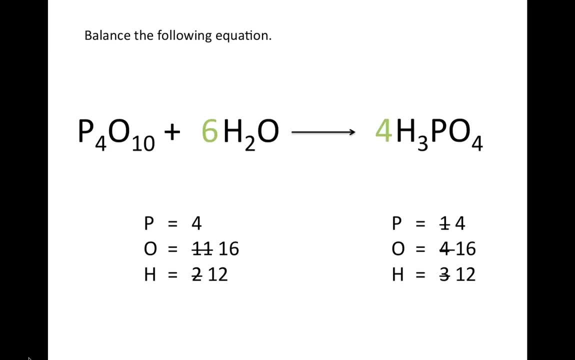 on the reactants. I'm going to do the same thing on the reactants and product side. This isn't always the case. Sometimes you need to go balance that third type of atom, but sometimes you'll be fortunate enough that it will just work out and save you a little less work. 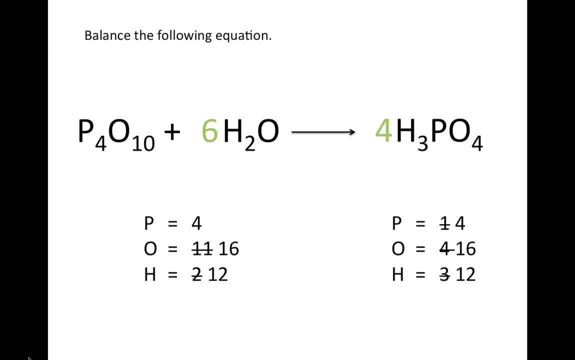 And now, because I have the same number of each type of atom on the reactant side and the product side, I can consider this reaction correctly balanced. Thanks for listening to Chemistry Solutions. I'll see you next time.